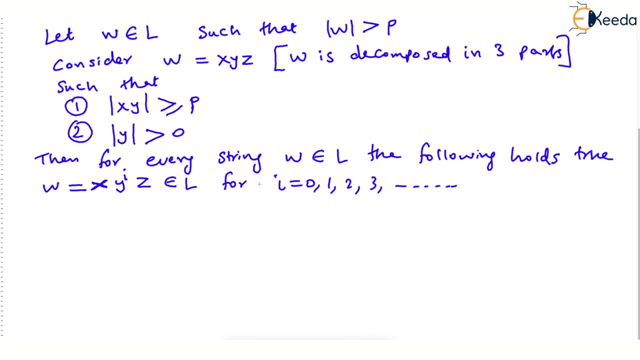 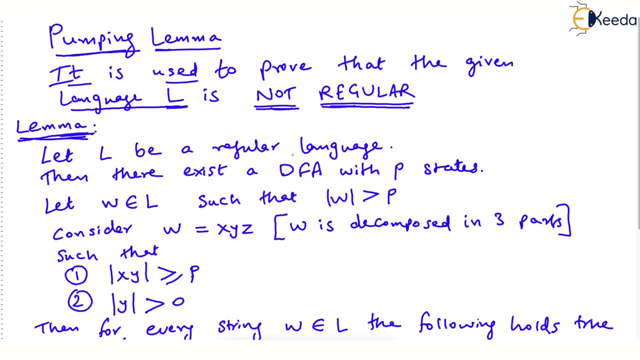 Because if the last step occurs as a contradiction, then it can't be regular, Something like that. This is known as proof by contradiction. So, repeating it, we actually want to prove that L is not regular, But we will start assuming that L is regular. Then you tell me if L is. 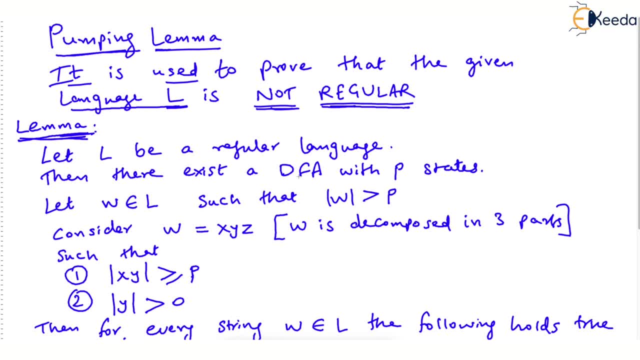 regular language, then surely there exists a DFA. Yeah, definitely. For any regular language we saw in the previous video, DFA must exist and DFA will have some states, let's say P states. This P can be anything: it can be 2, it can be 5, it can be 15 states, depending on the language. But if we assume 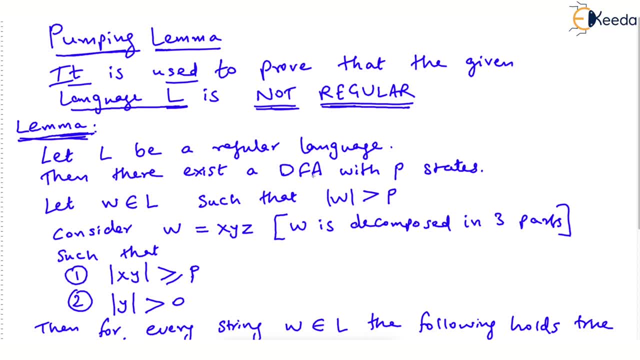 that L is regular language, then surely DFA will exist and it contains P states. let's assume Now, next part of the lemma says: consider some word, some string W which is element of L. Some language is given to us, then it that language will contain many strings which are element of. 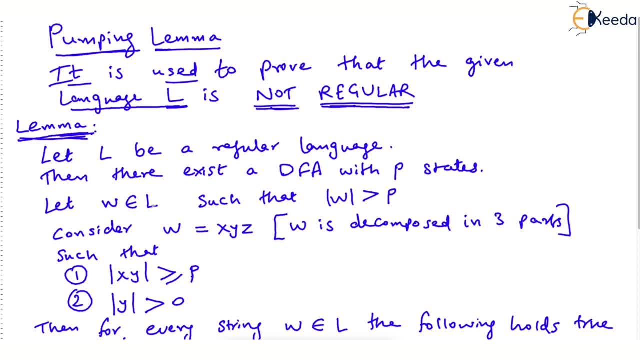 that language. Consider some word, some string which is element of that language. okay, but you consider such a word, such a word, whose length, this is length of W, the length of the string is greater than P, greater than number of states. The string that you consider from the language should be such: 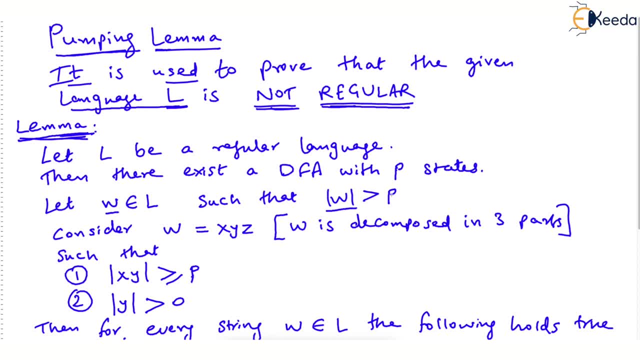 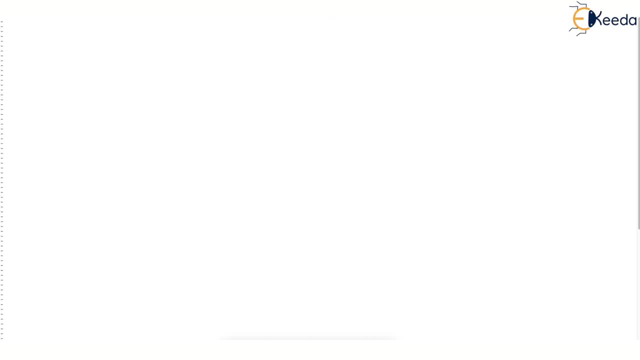 greater than length of the string should be greater than the number of states in the DFA. Here comes the point. One might wonder that if suppose, if we have a DFA, let's say, there is a language L. Just check this point. there is a language L of the form a raised to n, b, such that n is greater. 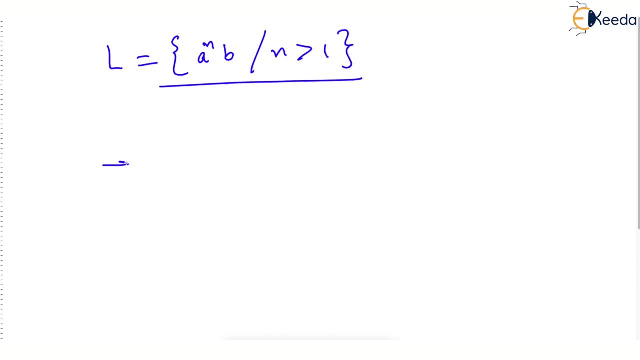 than 1.. You know DFA exists for this and a very quick. in the previous video we saw a very quick DFA That we constructed was a, followed by any number of a's, but last letter should be b and this is the final state. but after this last letter, if there occurs any other characters, we will send it to. 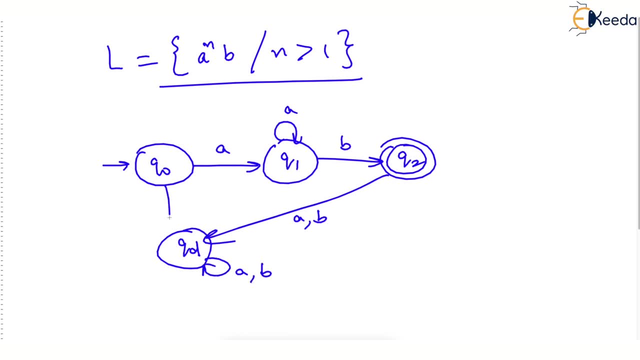 dead state where we will just toggle with a and b, and if the first letter is b one, then we will send it to final state. Now, how many states are there in this? The number of states? the number of states are four, including that state. number of states are four. That means 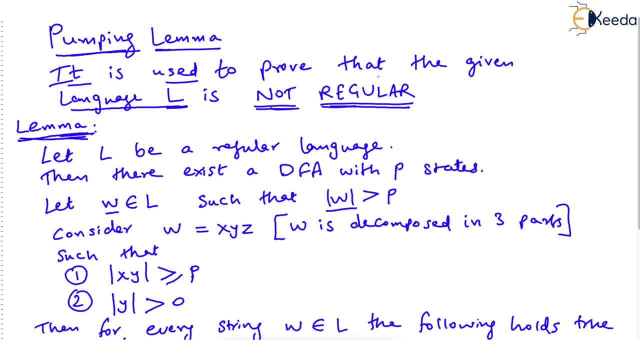 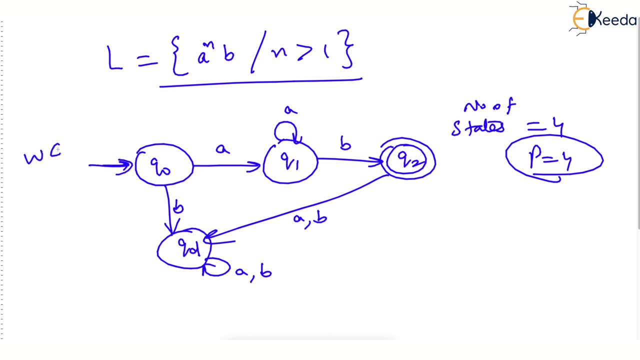 p is four here. Check this point: This p, the number of states, p for our DFA is four and given language L, we are assuming that it is regular. Okay, So p is four. Then can we give a string, w which is element of L, such that w length of w is greater than p? Yeah, definitely we can give a. 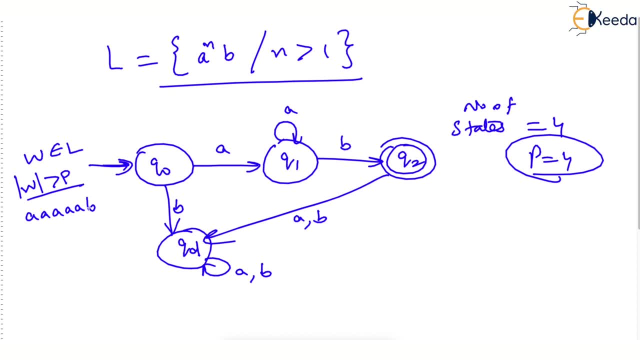 string like this: a, a, a, a, a, b. Check the length of this word, and this is the length of this word. This word is element of L, isn't it? Length of this word is indeed greater than number of states and you know the string will be accepted because after first a, we have a is repeated, so this loops here. 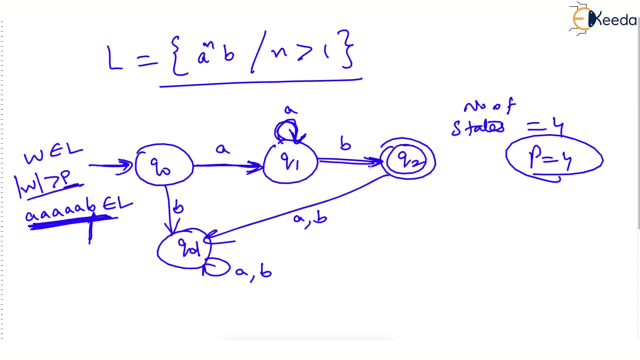 and then the last letter, as I am marking, is b, which will take us to final state. Hence, if w is element of L, then we can take a string where length of w is greater than p. I hope you accept this, because there are some loops somewhere in the DFA which will eat up. which will eat up. 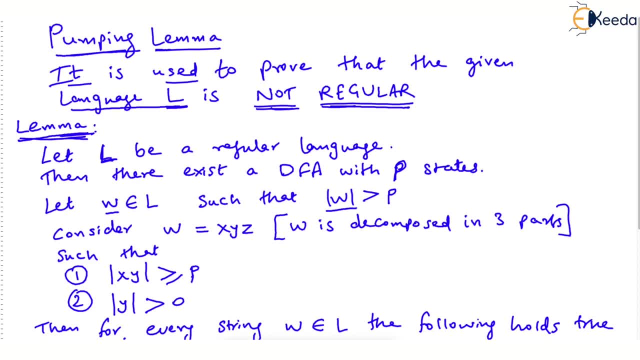 many letters of the string. Okay, So where were we in the pumping lemma is that you consider a word w which is part of L or element of L, such that length of w is greater than p. Okay, Now you think that this w which you are considered, you decompose it into three parts: x, y, z, As an 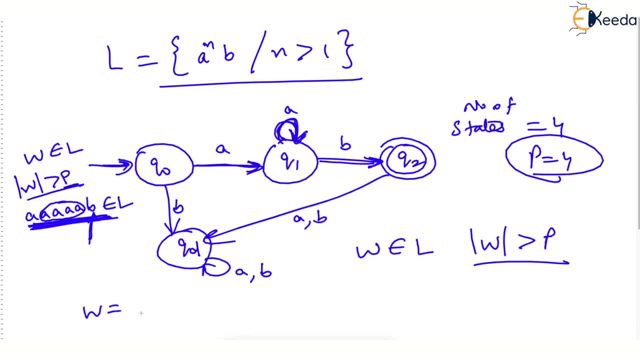 example, the string that we considered here, w, was considered as five times a and then b. this was w. think of that. you are decomposing it into, say three parts. this part is called x, this is y and this is z. or or you have got five times a and then b. you may say: this is x, this portion is y and this. 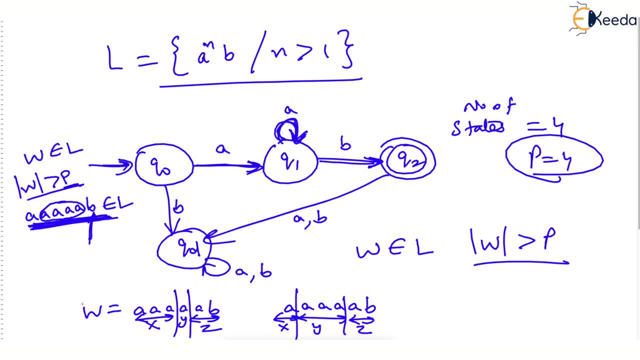 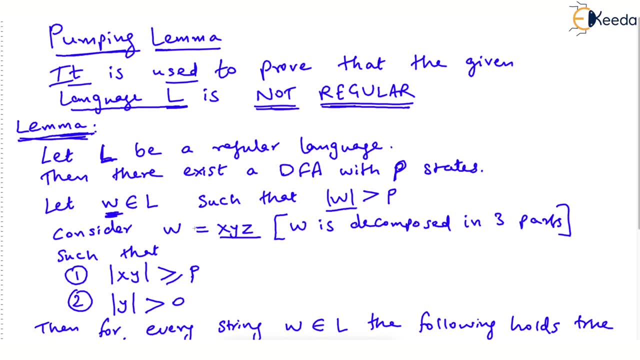 is z. Some way, you know some way, you decompose this w in three parts and call them as x, y, z. Okay, So think of this w decomposed in three parts. Okay, So think of this w decomposed in three parts. 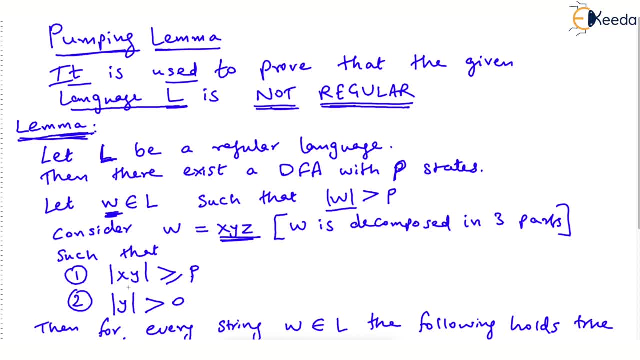 x, y, z, such that now these are the conditions- such that length of x, y taken together- this is read as length of x, y component taken together- should be greater than or equal to p of what is p, number of states. but length of y- only y, if you take- must be greater than zero. that means y cannot be empty y. 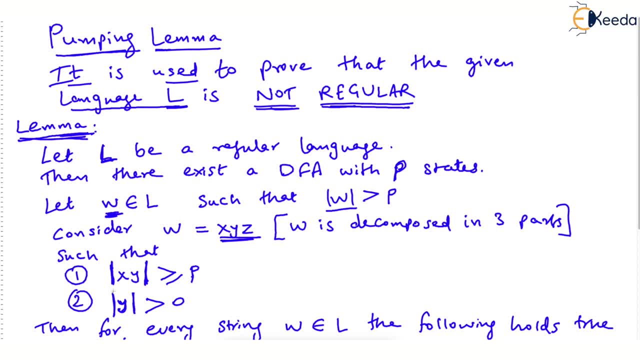 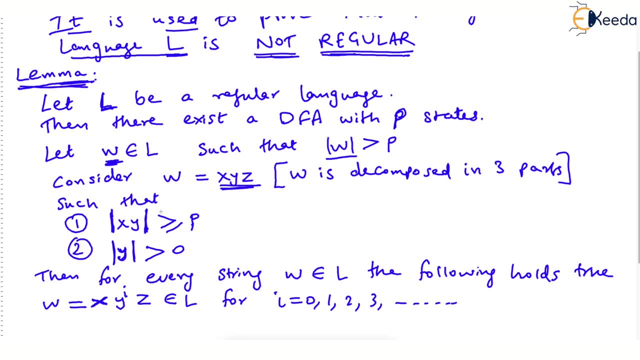 should contain at least at least one letter, because length of y is greater than zero. Okay, And then comes the last part of the theorem, which is actually the basis, which actually solves the basis, which, whatever considerations that we have done, we may get a contradiction here. 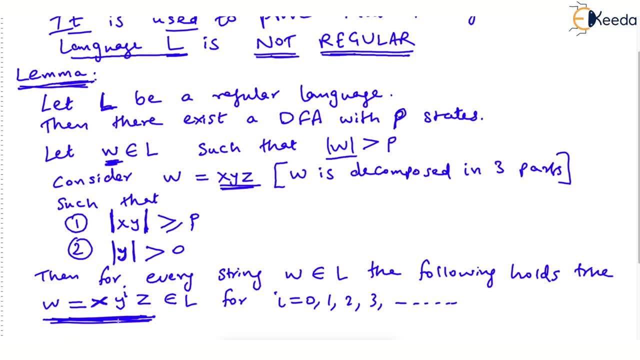 Okay, But have patience, We will learn what we will learn. this last point, what this last point is only after making the things very, very clear about what we have written earlier. So let's consider a problem like this: Prove that a raised to the power of a is equal to a raised to the. 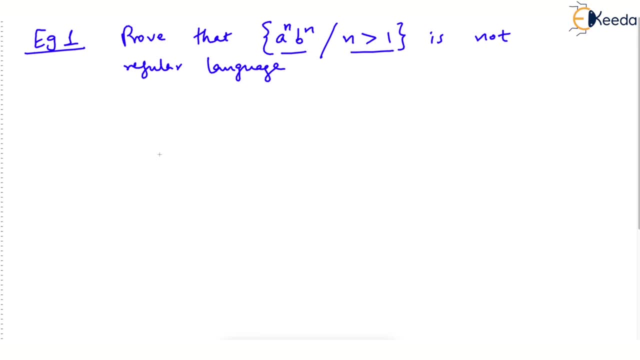 number of b raised to n and even when a raised to the power of a is equal to a, the relative number of b raised a to some entry in N on we will find n. These nestex functions, all these Hydroxylers here. 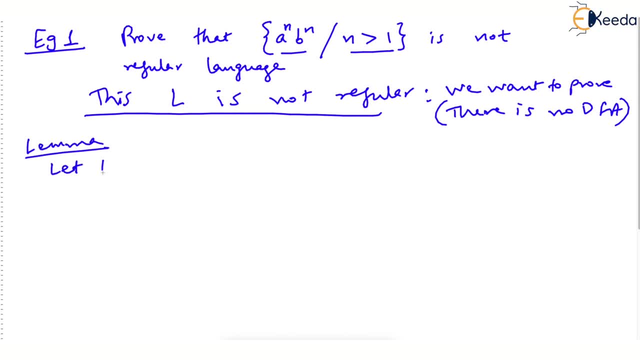 What's the way the funnels populate? Alright is equal to zero. The обычal same: Yeah Enough. let the given, let the given language, L be regular. So we start with an assumption that this language, a raised to n, b raised to n, n greater than 1, is. 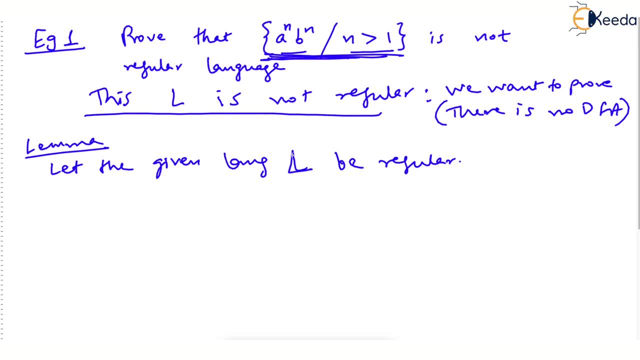 regular. So you tell me, if I am assuming that L is regular, then there exists a DFA, Then there exists a DFA, How many states in the DFA? Let's say that there are P states. There exists a DFA with P states. Now you might ask me, what is this P sir? Is P 4?? Is P 15?? What is it, Hello we. 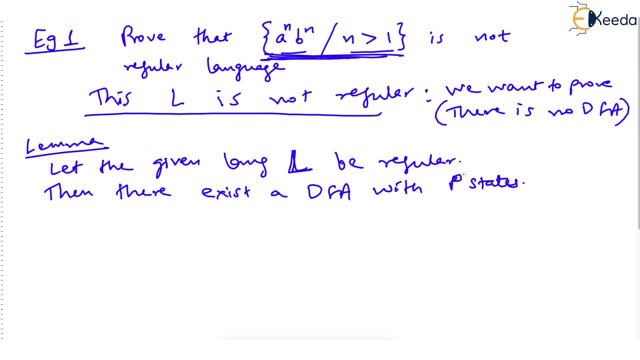 don't know, because we are assuming that somebody has made DFA for this language and that DFA contains P states. P is some number, it might be 40 states, it might be a hundred states, We really don't know- But we are assuming that there exists a. 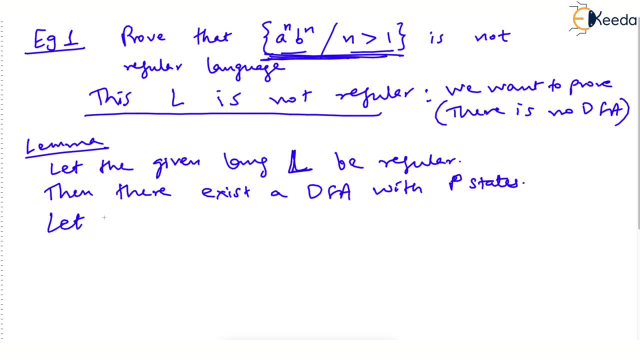 DFA with P. P states: now let us consider some W, which is element of L, okay, such that length of W should be greater than P. give me some strings which are part of this language. you tell me isn't W a comma B? yeah, this is part of the. 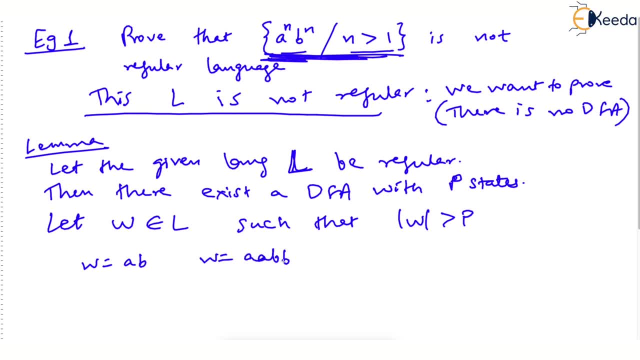 language. or W double a, double B- yes, this is also part of the language. or W triple a, triple B is also the part of the language. all such strings are part of the language, so you can consider any such string, any such string which is part of the language, but, but, but, wait a minute. wait a minute. you should consider. 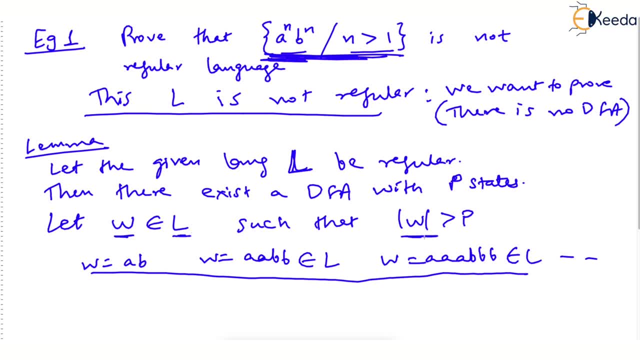 a word which is part of the language, but the length of the word should be greater than P, and P is the number of states. here is the most important point that you should realize while working with pumping lemma. which world should I take? should I take this word, or should I take double a, double B? should I? 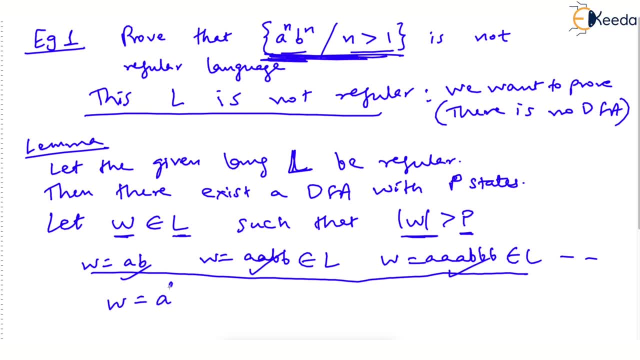 take triple a, triple B. what if somebody says: sir, take a cube B, cube, triple a, triple B, because it is element of L. but then are you sure? are you sure that that length of W is greater than P? what is length of W here, by the way, six, three A's. 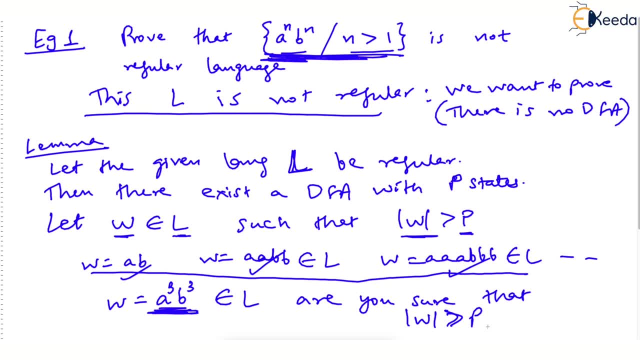 and three B's, six is the length. then are you sure that length of W is greater than the number of states? you would say: how do I know, sir, because I don't know P. what is P? who knows that the DFA constructed with P states this P might? 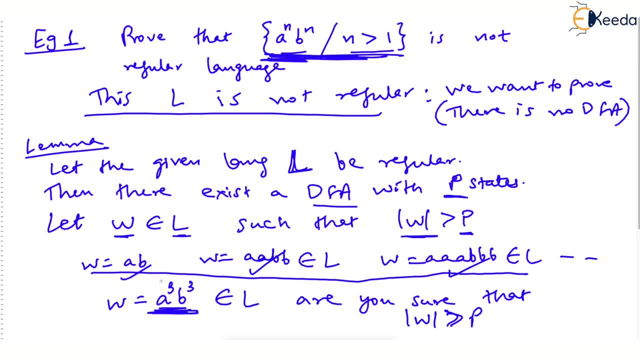 be 40 states. so you would then say, sir, take a raise to 40, B raise to 40, now the length is 80. then now, definitely, length of W, which is 80, is greater than P. but we really don't know P, we don't know the value of P. how many states are there? how? 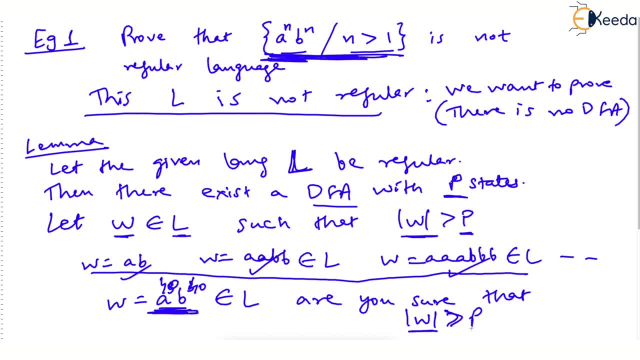 can we claim that some particular string, you, which is part of the language, will definitely have length greater than P? I hope you are understanding my problem. what I am trying to explain is that the big, big point about this theorem is that you take some word, some word which is: 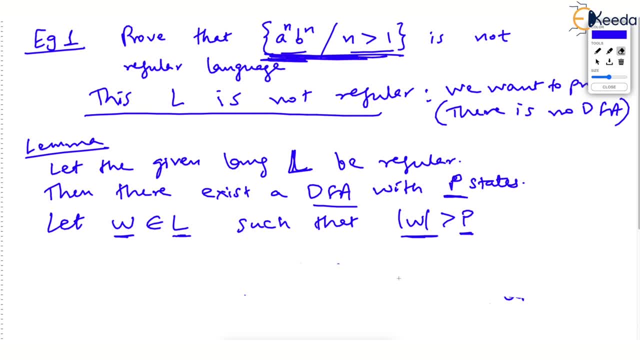 part of L, but make sure that the length of that word should be greater than P. so which word you should take where you can be hundred percent sure that length of word is greater than P? here comes the word. we can take the word as a raise to P. 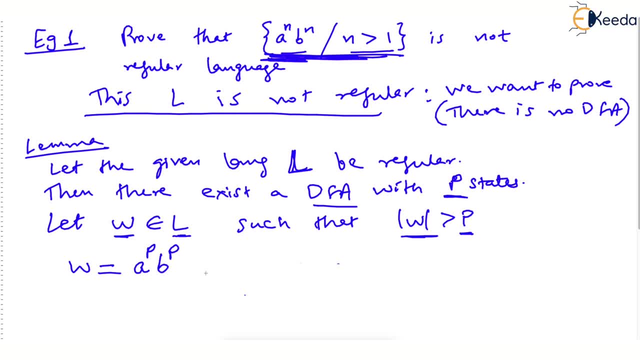 B raise to P. what do you say about this? what kind of string is this? how many is are there in the beginning? he is, and how many bees are then pbs. so you have W as a repeated, a repeated how many times, p times, and then be repeated, be repeated. 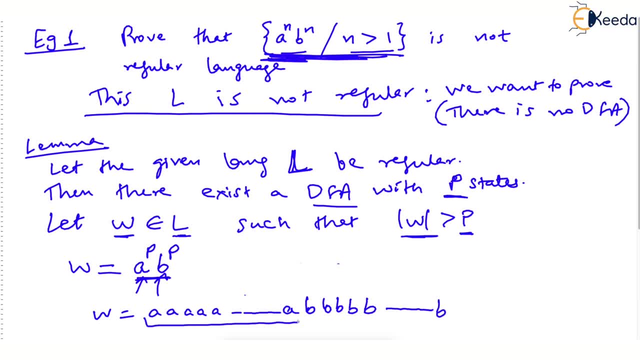 how many times p times? this is exactly P number of A's and this is exactly P number of bees. is a raised to p, b raised to p? and this is part of language. come on, this is part of language and we are also sure, surely, surely? length of w is greater than p, because length of w is now 2p. 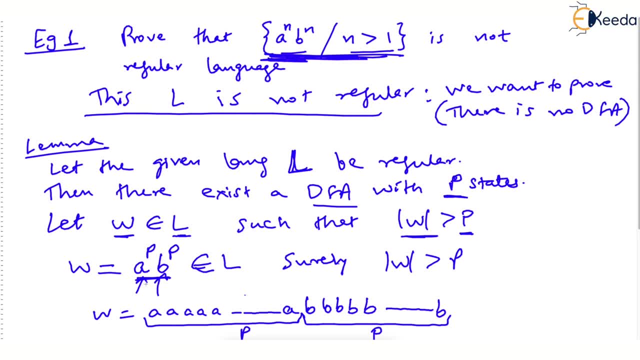 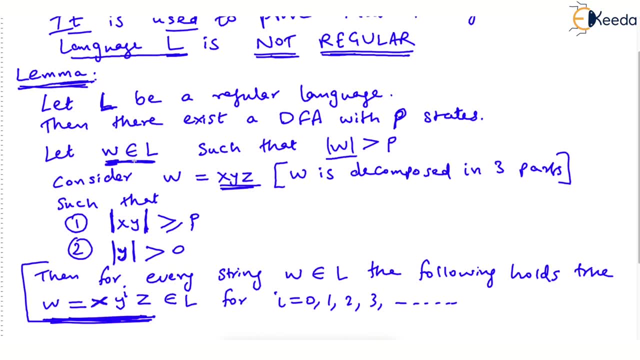 2 times p. you can be now sure that this is what we want, as far as the lemma says. the lemma says: take some string w, which is element of l, but length of p should be greater than- surely greater than p, and we have taken such a string. now the next part says that decompose w in three parts. 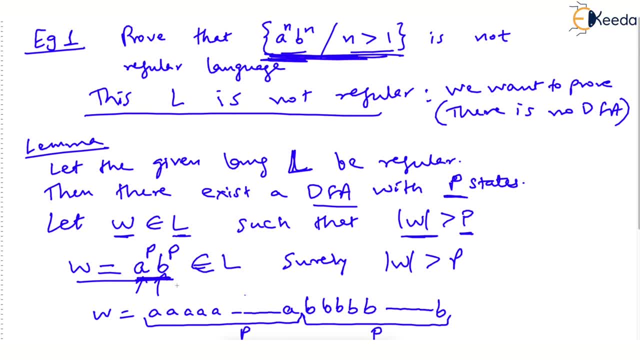 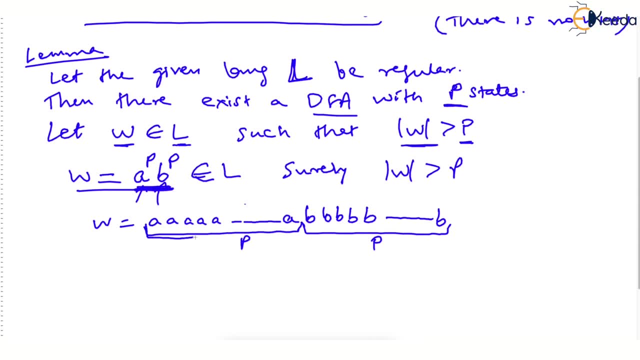 x, y, z. now watch the string that we have taken. check this. this is the string: a raised to p, b raised to p. there are exactly p a's in the beginning and p b's at the end, so the length of this is 2p. we want to somehow decompose this into x, y, z, three parts. 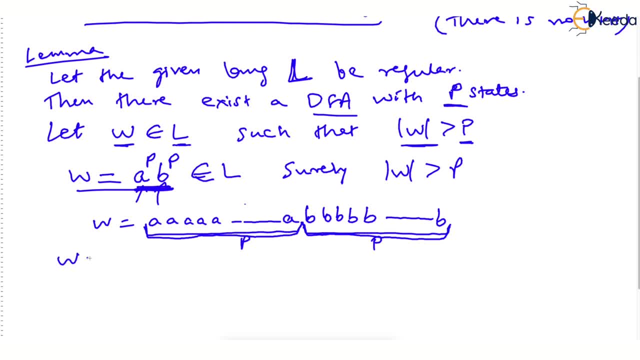 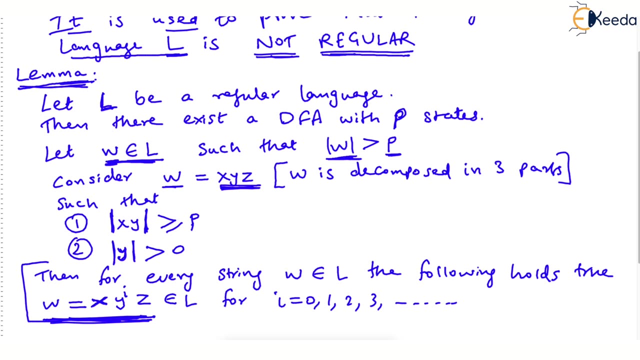 but then there is a condition: w should be decomposed as x, y, z, but the condition, first condition- is length of x- y. length of x? y should be should be less than or equal to p. let me check if i made some mistake. oh, this should be greater than or equal to p. wait a minute, i have written. 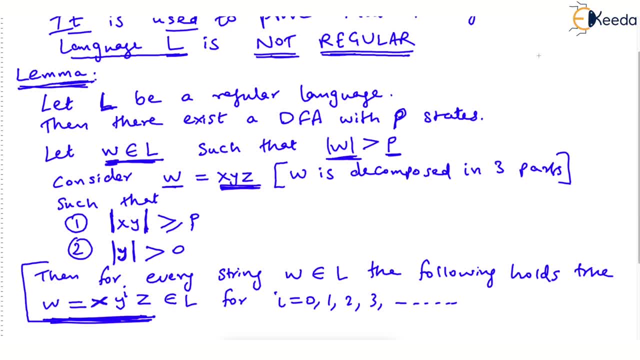 this less than or equal to. i made a mistake here, just check. this should be: this should be less than or equal to p. i'm so sorry. x y be less than or equal to p. okay, So this is the condition. You tell me if x y component. 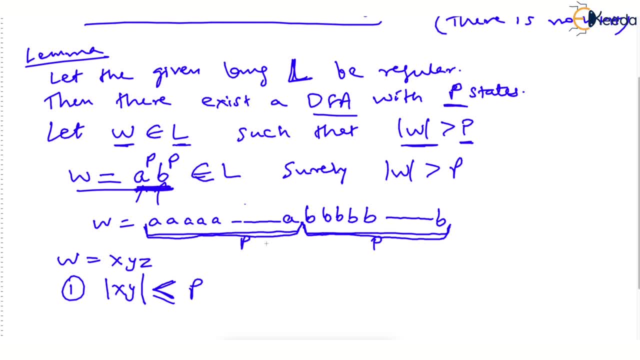 has to be less than or equal to p. then if we break this, if we break this particular string, w into x y, z into x y z, three parts, then x y together, x y together can. 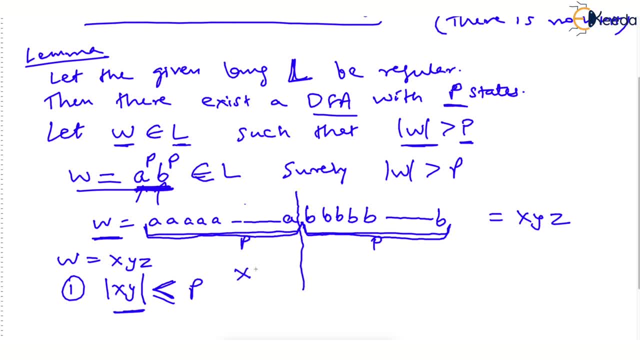 be at most up to this point. x, y together can be at most up to this point, because this length is p. That means y cannot be after this a and this part can be z. I repeat: when you decompose this w into three parts- x, y, z- then length of x, y taken together just. 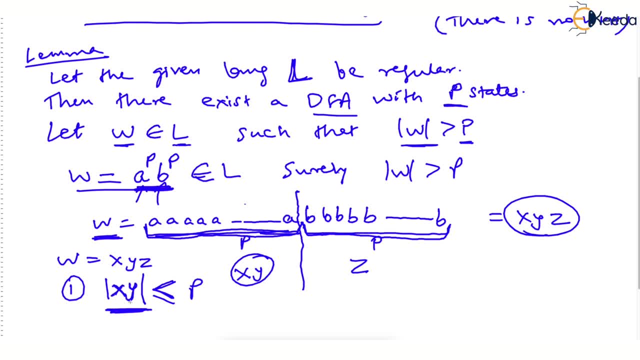 notice: x is one part and y is other part, But if you take them together their length collectively should be less than or equal to p. So maximum part in which x, y can span is this: p characters, because length of this much is p. 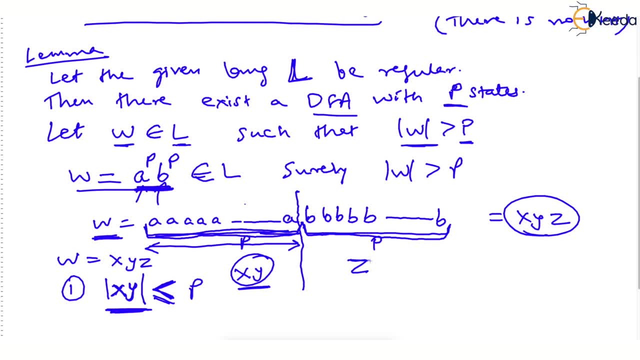 So x, y can be at the most up to this point and next will be z, Or or. we can have, if w is a is a is repeated p times and then b is b is repeated p times. Check that These. 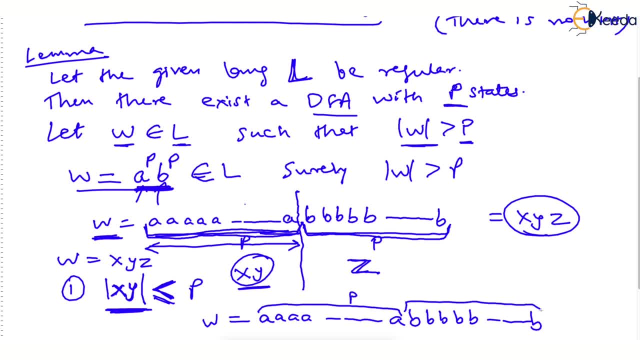 these are p? a's and these are p b's. Then you can. you can say: this portion is x? y, Why not? You can say: this portion is x? y. Tell me what is the length of x? y now, Well, 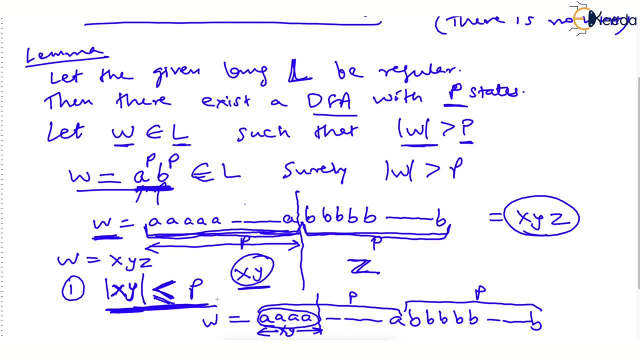 less than p. yes, less than p, That's also allowed. Then all this part is z, But length of x, y should be less than or equal to p. Please try to understand, Okay. So how are you going to decompose this string? Give me some time. I'll just redraw this string again. 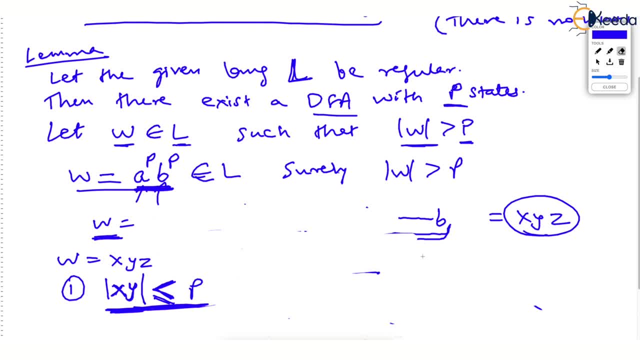 so that we see how we can decompose One way of decomposing, one way of decomposing so that we preserve the rules We have a-relative A repeated a repeated p times, then b repeated b repeated p times. Correct This much this. 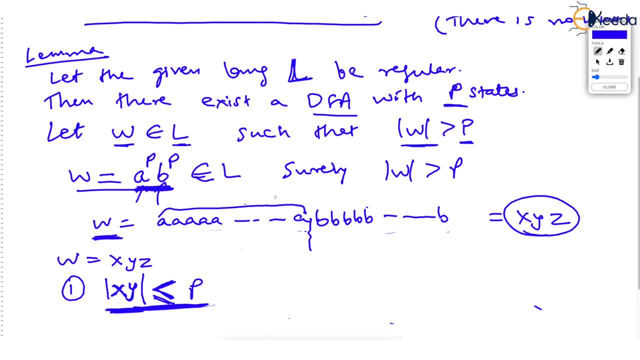 much is length p. Just check: This much is length p. What follows is exactly p number of b's. What if we take this much as x y, This much as x y? Then the rule is satisfied because length of x- y together is p and it can be exactly p also. 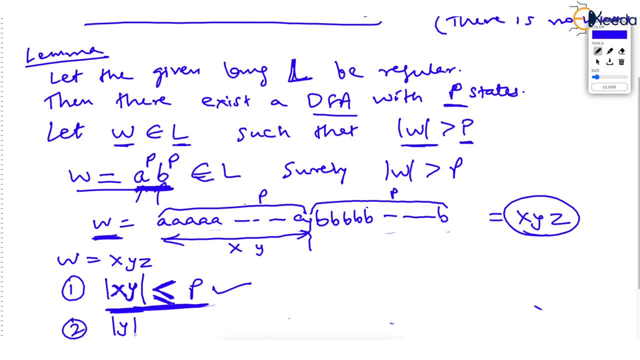 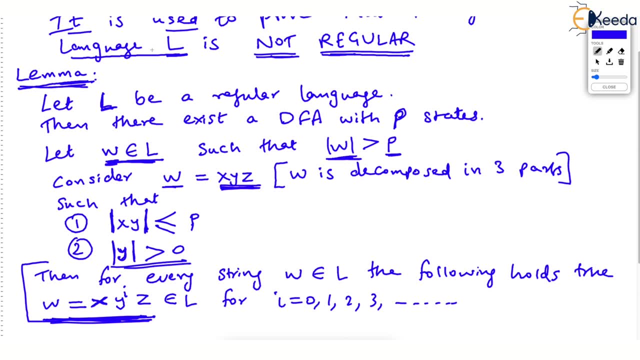 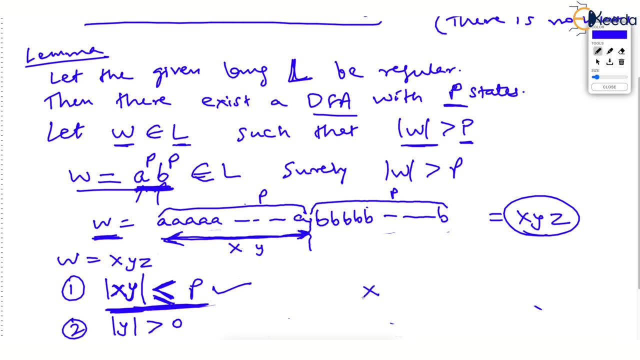 But the second rule states that length of y component should be greater than zero. Check the second rule while you are taking this. Length of y should be greater than zero. That means we have considered this entire portion as xy. Now let's think of what should be x. 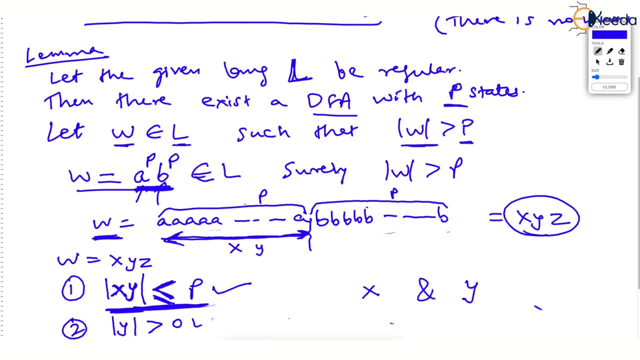 and what should be y. Length of y should be greater than zero. How about saying y you b in this region only, but y u b a single a. Still, you see, x and y very much coincides. Let's continue. 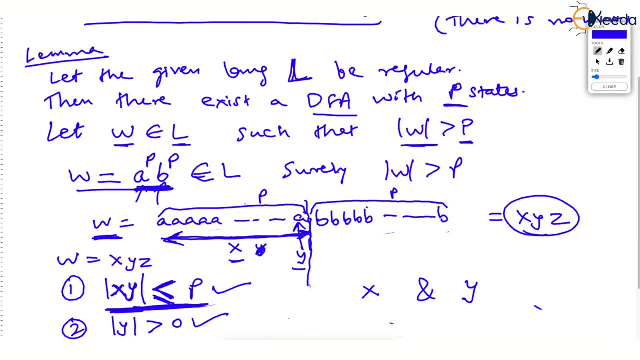 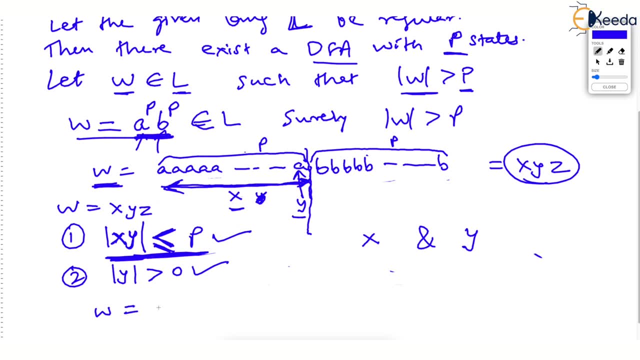 Y collected together is exactly P P letters. So I guess you are understanding that we have decomposed W in this form. We have decomposed W, X, Y, Z as follows: We have exactly P number of A's and exactly P number of B's, but we are calling this as Y, only single A as Y and these remaining 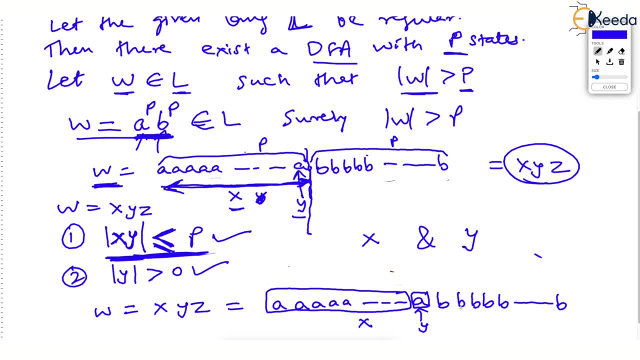 A's here we are calling them as X, and rest of these all B's, we are calling them as Z. You just tell me, if X, Y is taken collectively, what's the length? Come on, length is P, and first rule is: 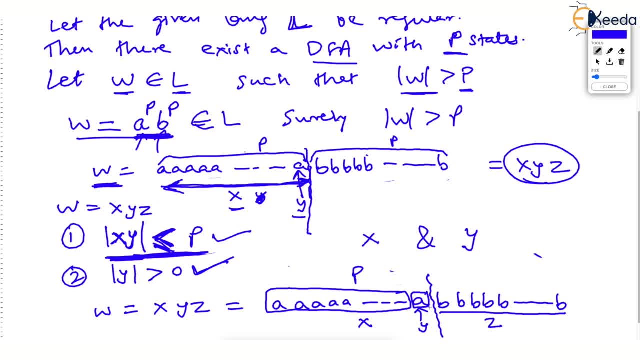 satisfied. and second rule is also satisfied because length of Y should be greater than 0 and it is greater than 0 because length of Y is 1.. There is one A in this section. There is no rule for Z. There is nothing written. 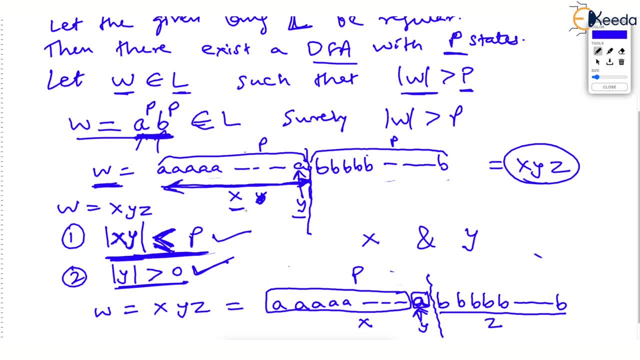 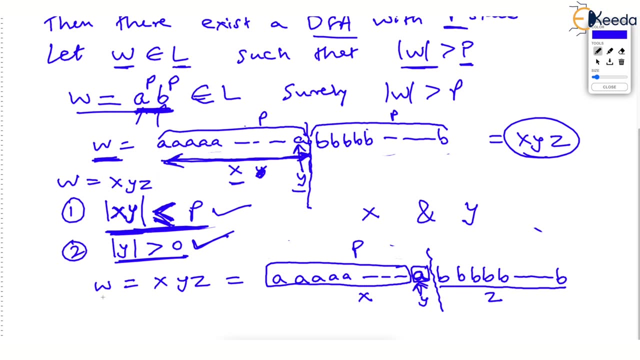 About Z. Z can be the remaining component. and now the last point: Just check, We are really driving ourselves to complete this. Now, what last part says is that you try to find out or figure out or generate new strings from this given string, Taking X, Y, Z, as you have shown here. 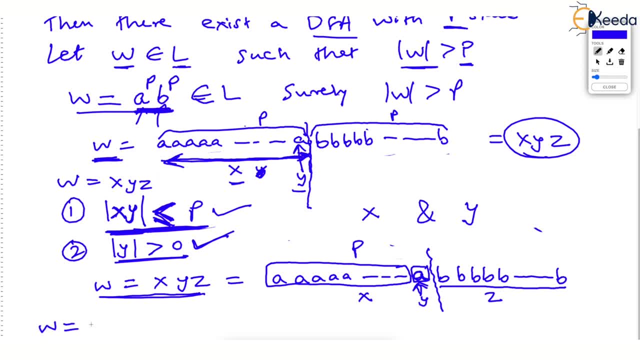 taking X, Y, Z, you generate a new string. Let's say a new string is X, Y raised to 2 and then Z. Try to understand: Y raised to 2 means you are repeating Y component 2 times. What will be the? 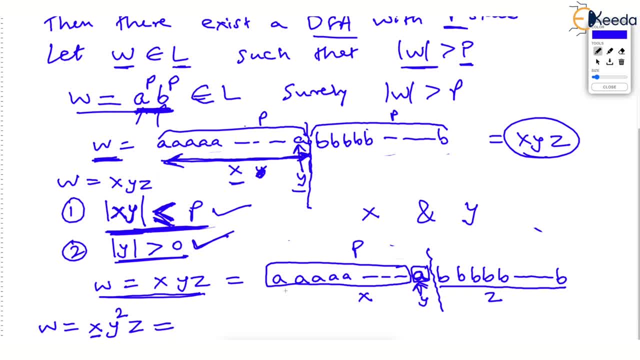 new string. Tell me what is X. Oh yes, X is all these A's. How many A's are there? A's are P minus 1 A's. So here we will write X unchanged. X is P minus 1 A's. This is X in the string W. but 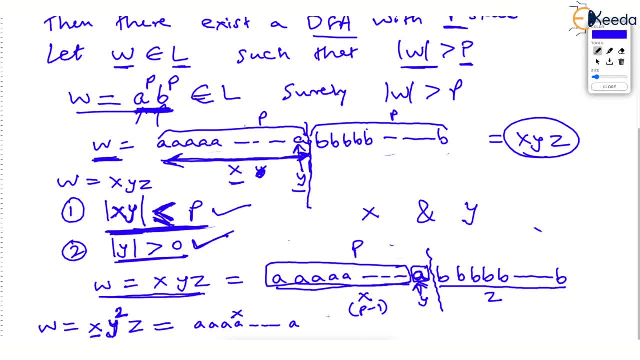 it is saying that Y should be repeated 2 times. What was Y? Y was single A and we have to repeat that Y 2 times. This is Y square. Please try to understand. And then Z has to be written as it was. Now. notice: Z had exactly, exactly P number of these. Now what's the new string you have got? 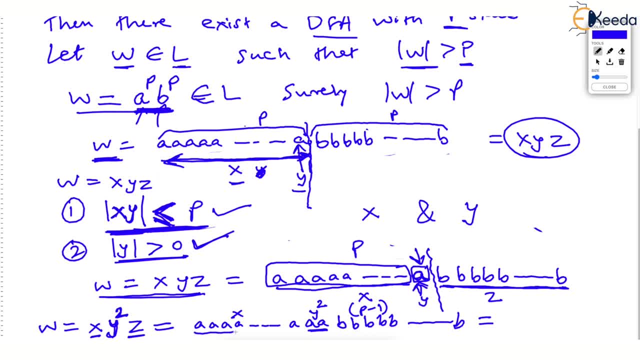 Be careful, be careful. What's the new string? How many A's are we having now? Check, check. How many A's are we having Previously? how many A's we were having P, But now we are having P plus 1 A's. 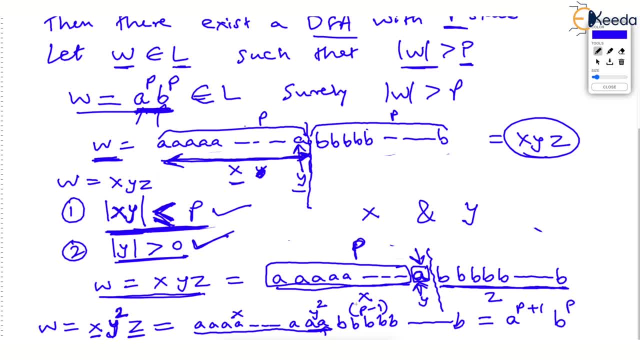 added here. But how many B's are we having? Still, the number of B's are P, because there is no change made to the number of B's. But this string, the new string that we have got, generated a new string by repeating Y. The new string that we have got is not the element of L, Is not the element of L. 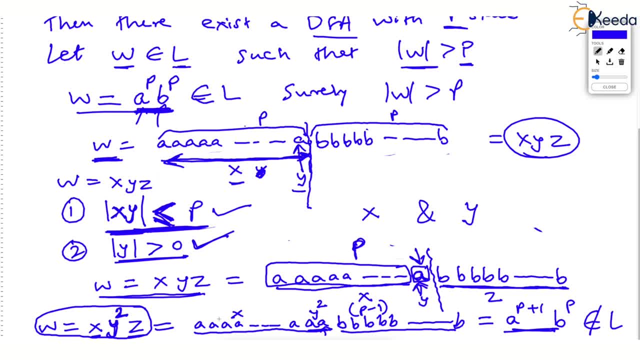 And notice, if the language has to be regular, then this new string also should be element of L, But it is not the element of L because number of A's are not matching number of B's. Then we have reached a contradiction And we have reached the contradiction, So we say that whatever was our 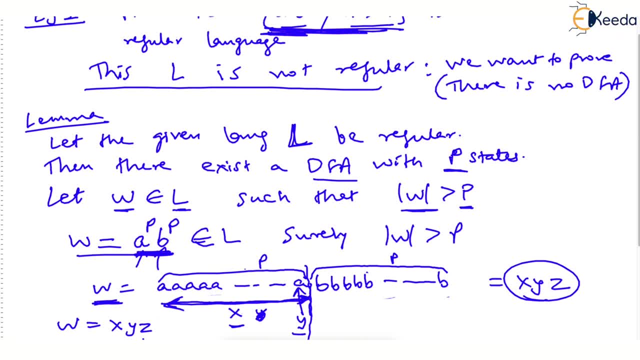 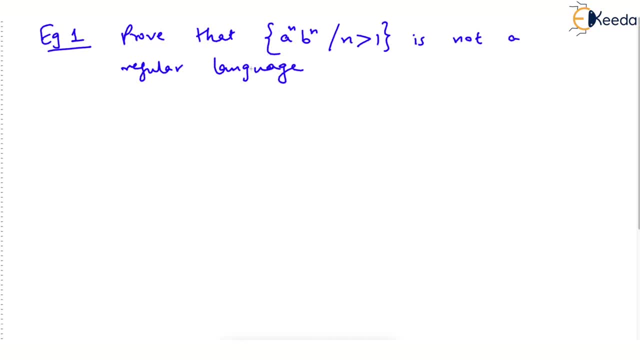 assumption. what was our assumption? by the way, Our assumption was that, given language, L is regular, So our assumption is wrong and the language is not regular. Be with me. Same problem, I am solving Same problem, But I will not write so many steps. Okay, Let's say language is regular. 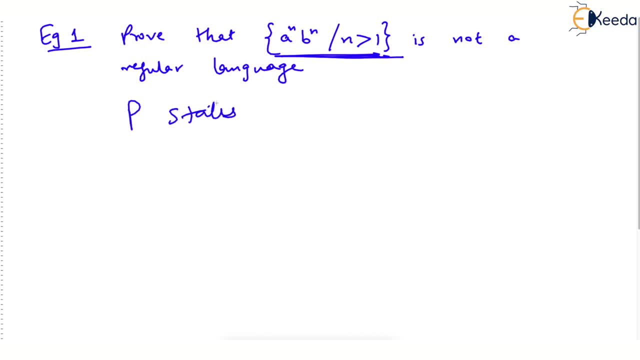 Then DFA exists And number of states are P states. Let's say DFA has P states. Let's consider W as A raised to P, B raised to P, which is element of L, And surely, surely, length of W is greater than P. 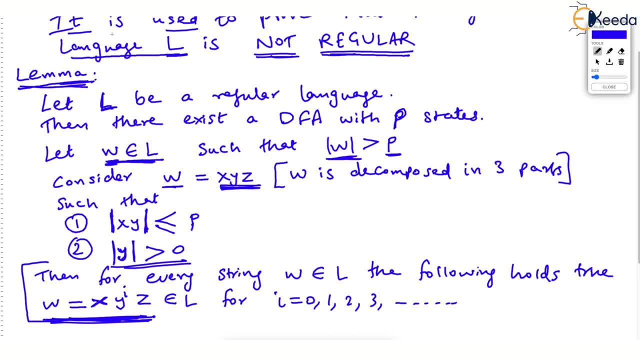 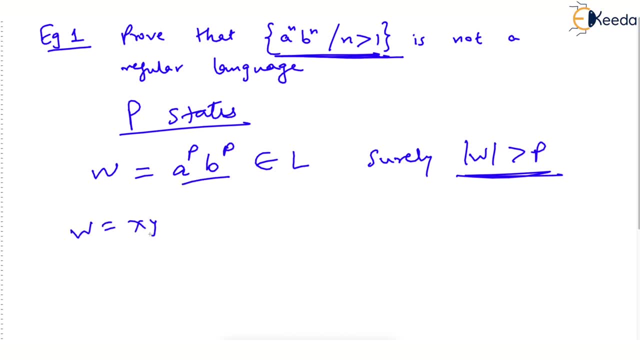 Definitely So. first rule, first suggestion is satisfied. Now we want to decompose this word, this word, into X, Y, Z, Correct, Such that length of X, Y should be less than or equal to P. But this string is nothing but number of A's are P A's and number of B's? Number of B's are P number of B's. 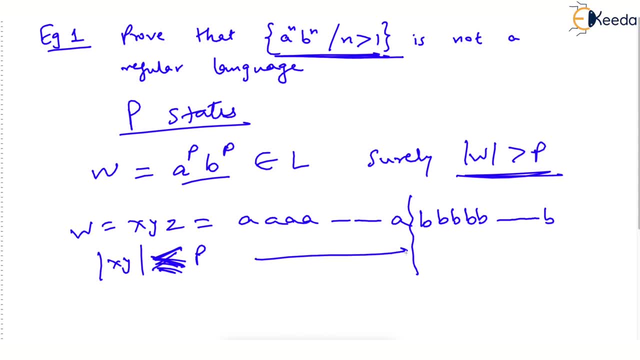 What if we say that this component is X- Y- Some repetitions here, Just mind it. This part is X- Y, Then surely the length of X, Y is less than or equal to P, because these are P number of A's. 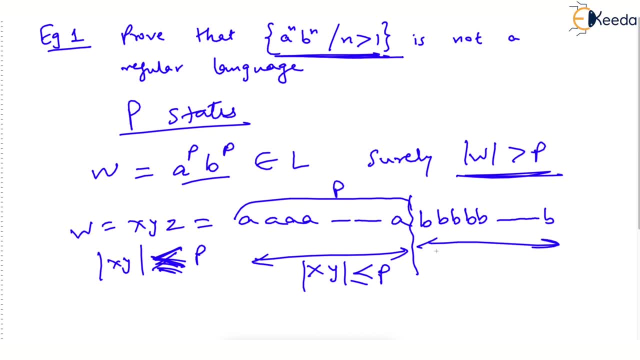 So we can consider this as X, Y and remaining as Z. But then if you say that this together is X- Y, you can say: this portion is Y, Only single A. Only single A is Y, Because the another rule says Y. 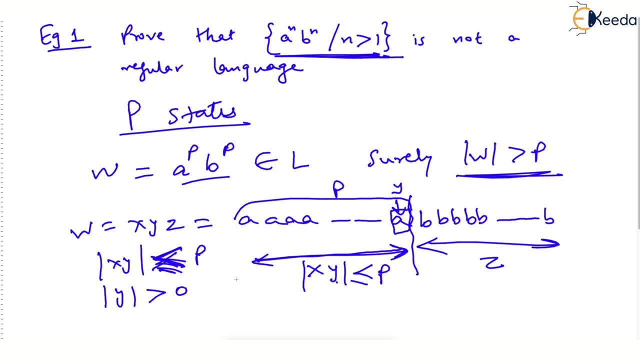 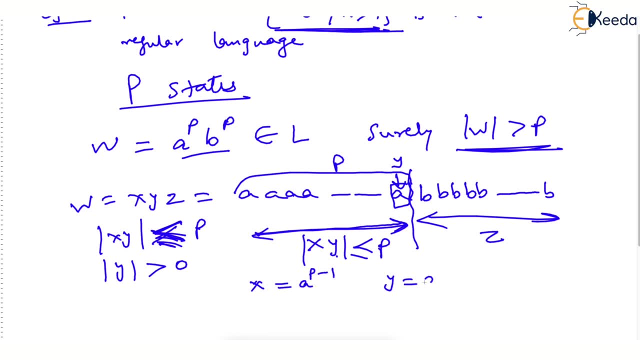 cannot be empty. Y should be at least greater than zero. So what exactly is X? X is A raised to P minus one. What is Y? Y is single A. And what is Z? Z is B raised to P. Now, what if you generate a? 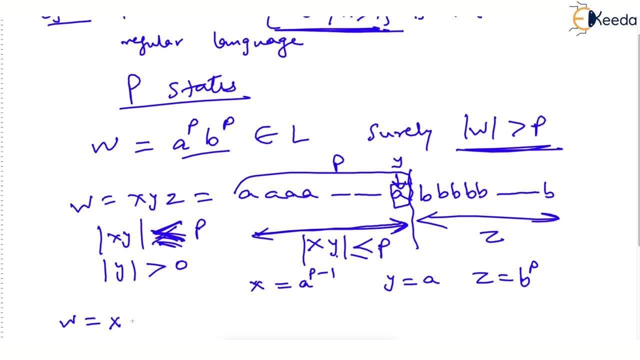 new language as follows. as follows: just check: X, Y, cubed Z. X, Y cubed Z. This should be element of L, But what is this new new string? X is A raised to P minus one. Just check this. But Y is repeated three times. Y is single A, So we'll get A cubed, Correct? 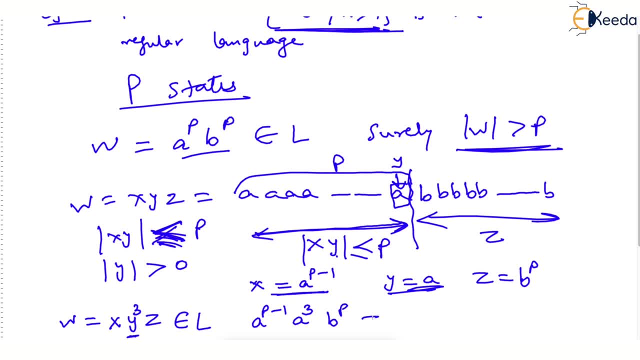 And then Z is B raised to P. What's the new string? Watch that this new string is A P plus two raised to P plus two. Check this. Followed by B raised to P, which is not the element of L. We have reached a contradiction. This should be element of L, but this is not the element of L. 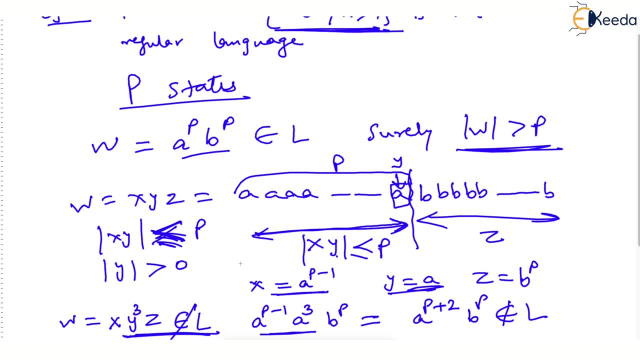 So the given language is not regular. I hope you are understanding the word pumping, What we are pumping. you know we are pumping as many Ys as possible, Pump in extra Ys, extra Y And, after pumping extra Y, if we are getting a new string which is not the element of L, 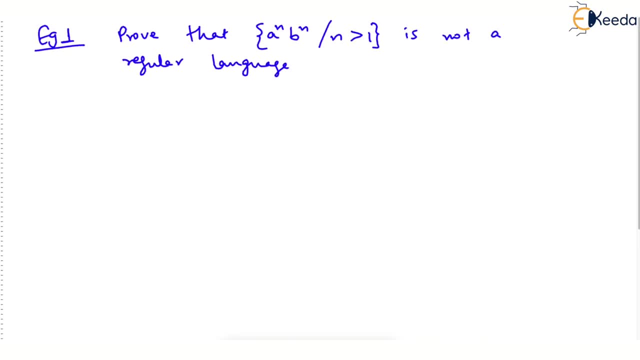 then we say that the language is not regular. Keep checking, Keep checking. Hello, Have patience, Keep checking. The same problem I am taking. Let's say DFA exists, DFA with P states And the language is regular. Let's say: 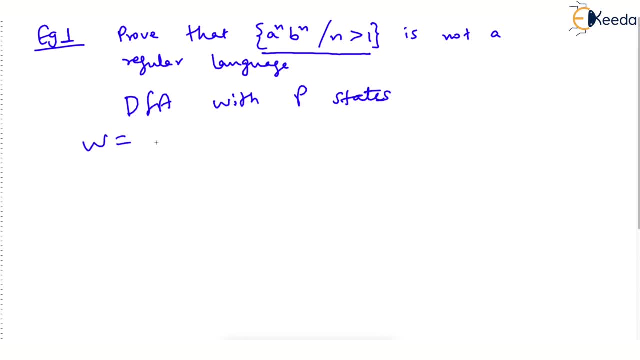 Okay, P states. Then consider some word: A raised to P, B raised to P. This is element of L and surely length of W is greater than number of states. Try to decompose W into X, Y, Z, But length of X, Y. 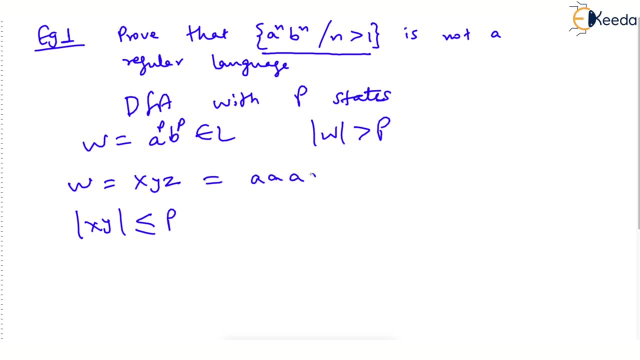 Should be less than or equal to P. Now this string, as you know, is: number of A's are P A's and number of B's: Number of B's are P number of B's. This much is the length P, followed by this much is the length P. 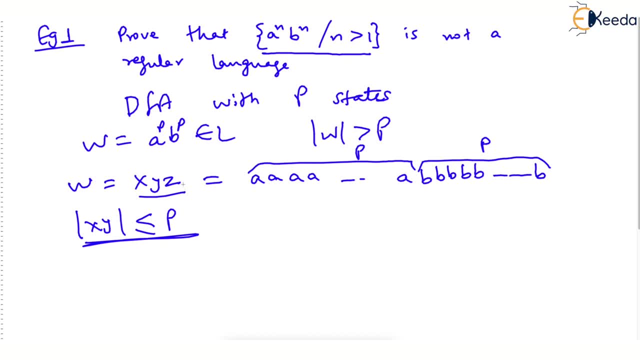 Now, length of X, Y in the decomposition should be at the most P. It can't be more than P. It can't be more than It should be less than or equal to P. Then how about saying this much: section is X, Y and this portion is Z. 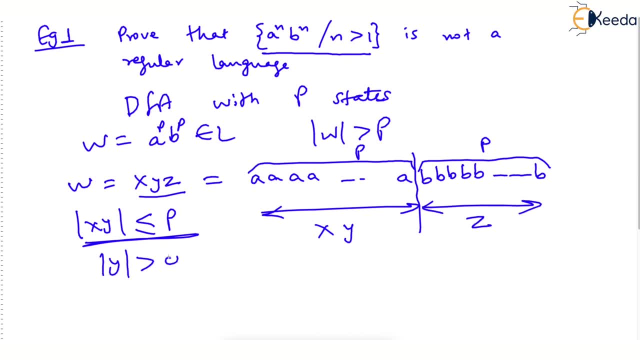 But another rule says that Y should be greater than 0. Length of Y. So why don't we say in this section only: this is Y. Still, you see together X, Y. If you take X, Y together, the length doesn't cross P. I hope you are understanding. 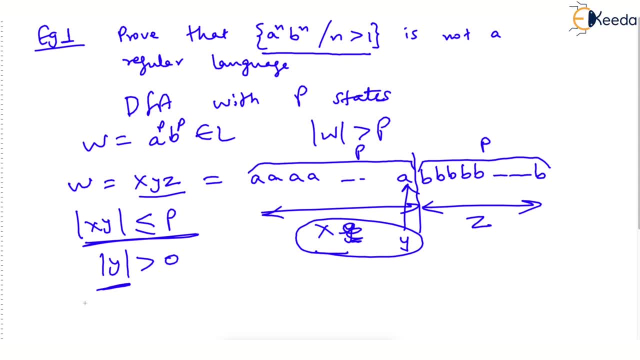 So now what if, By the way, what is X, X is A raised to P minus 1.. What is Y, Y is A Single A, And what is Z, Z is B raised to P. Now, what if you consider a string: X, Y raised to 0, Z? Look what you are doing: You are not pumping in Y, but you are pumping out Y. 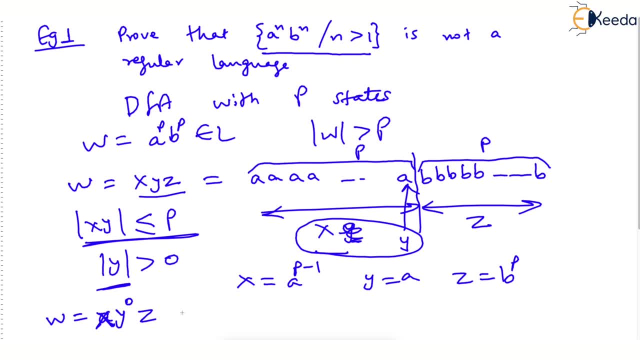 You are taking out Y. Y raised to 0 means you don't want Y component. What this string will be, X, is A raised to P minus 1.. And then you are dropping Y. You see Y raised to 0. So you will directly have B raised to P. This is Z component. 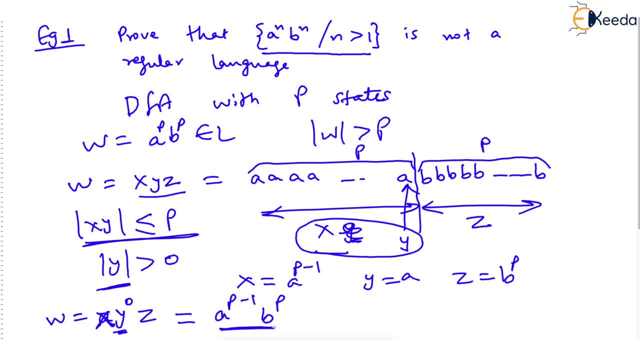 You have dropped Y, But is this element of L? No, Because number of A's have to be equal to number of B's. Listen, the strings are of the form A raised to N, B raised to N. This is not the element of L. So we have reached a contradiction: that DFA does not exist And this language is not regular. 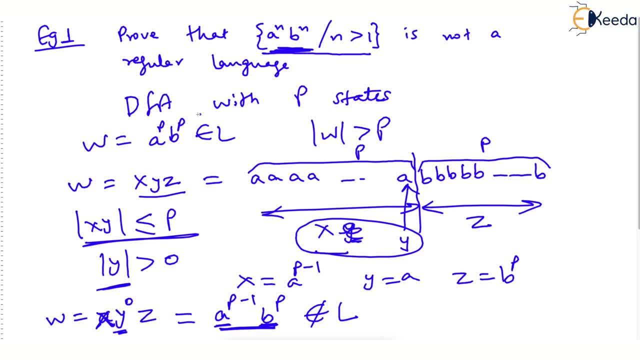 You know all the art, all the art of pumping lemma lies over here. Which string will you consider? And then decomposition will be ultimately understood, Trust me. But it's the art to consider a correct type of string whose length is surely greater than P. 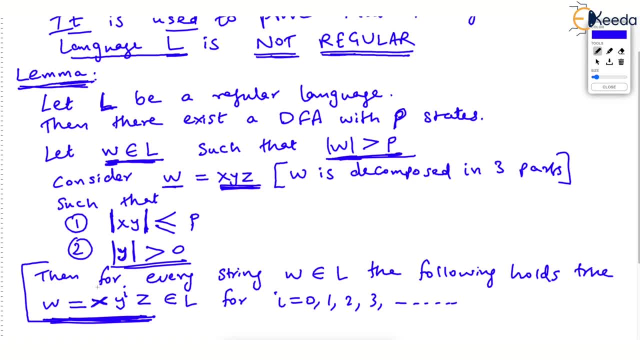 Now come back to the theorem. I hope you are now understanding the last line. Then, for every string W which is element of L, the following must hold true. The following must hold true: What is that? If you generate a new language- X, Y raised to I, Z, it should be element of L. 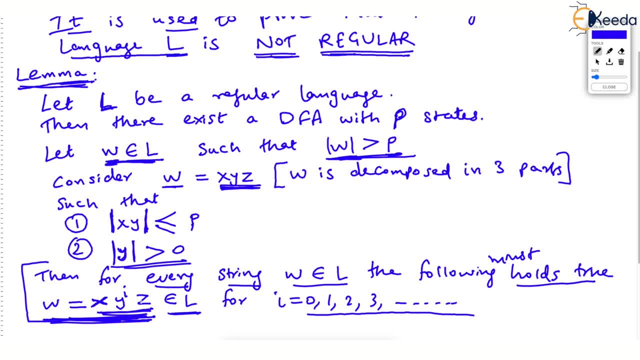 For I, running from 0,, 1,, 2,, 3 onwards up to infinity. You can put any I over here, Like we proved it with Y raised to 0, or we proved it with Y square, Isn't it? Yeah, we proved it, But then you see, this must be element of L. 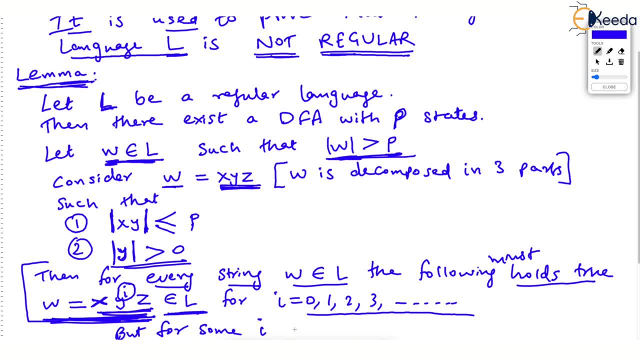 But some I, for some I. if W is not element of L, then L is not regular, Then L is not regular. Just see, the nice part about this theorem is, although it is written, I is equal to 0,, 1,, 2,, 3,, 4,.